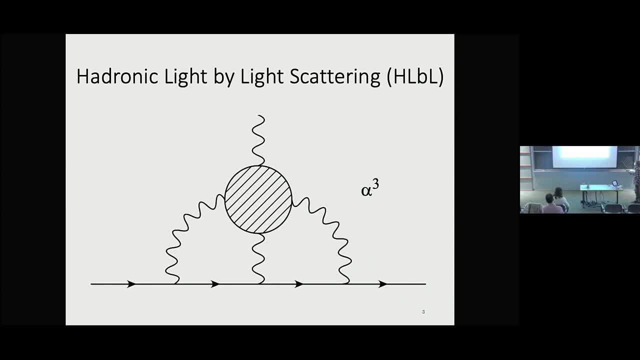 it's easier to get out of the way. This is sub-leading in the fine structure because there's three photons connecting the hadronic blob, But the size of the hadronic contribution from light-by-light is about the size of the current discrepancy between theory and experiment and the uncertainty is pretty large, or was 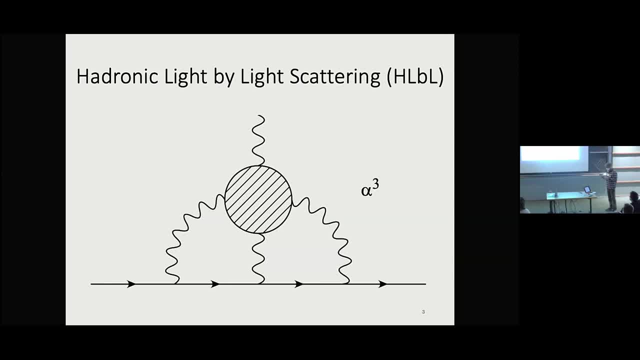 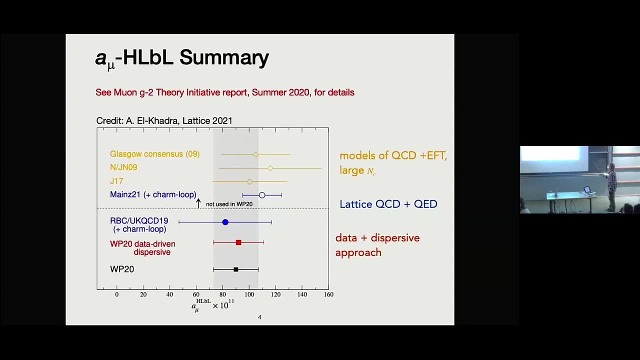 pretty large, So we have to make sure that we have this under control, And the good news is it seems to be under control. So for a long time we used what's known as the Glasgow consensus for the hadronic light-by-light contribution, which was based on models and effective field theory. 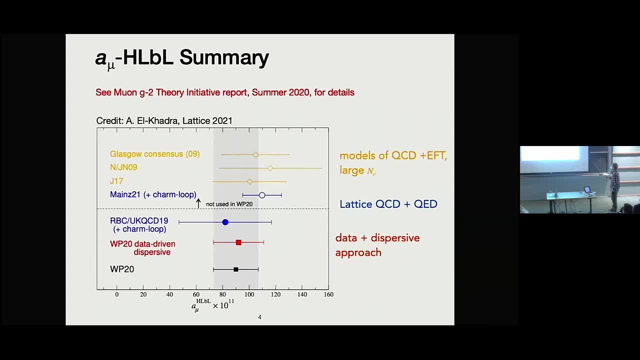 But now there are data-driven approaches, just much like the hadronic vacuum polarization, and the errors are really under much better control. And we also have first principles, lattice-QCD calculations, And if you take these two into account, and so this is from the muon g-2 theory initiative, 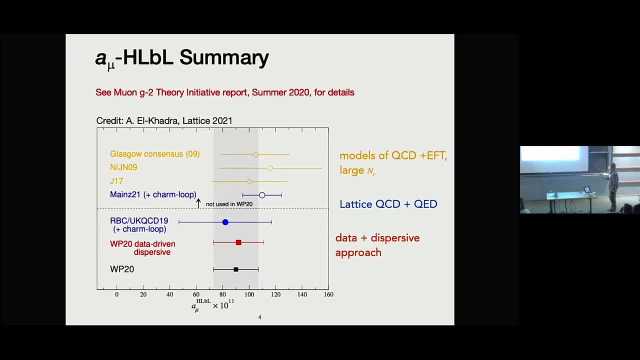 white paper in 2020, then you get this answer for the hadronic light-by-light contribution. So I'm going to stop there, Thank you, Thank you. And so we have, as I said, hadronic light-by-light contribution. 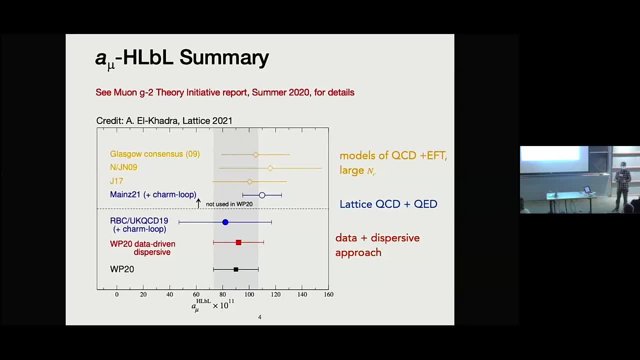 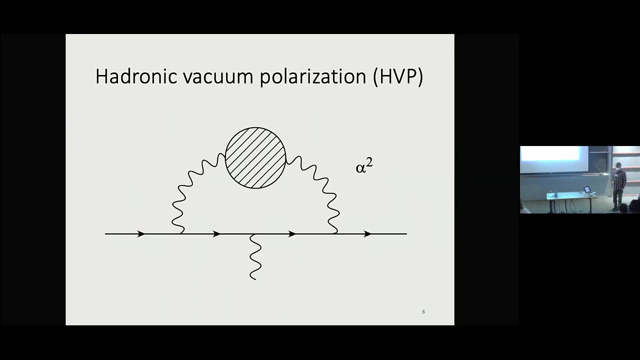 And what this means is that, basically, light-by-light's not going to solve our problem. It's not the reason for an apparent discrepancy- if there is one- between theory and experiment. OK, So now let me move on to the hadronic vacuum polarization, which is the leading hadronic 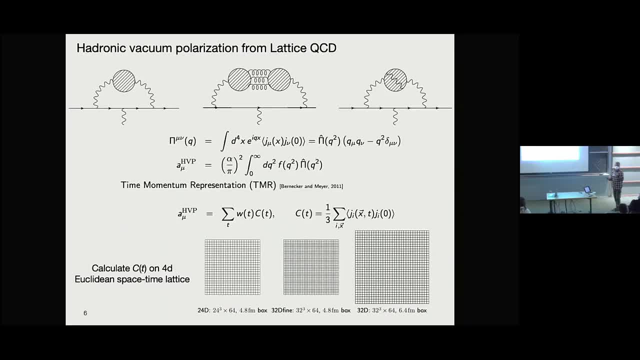 contribution. So most of you are probably used to, you know, calculating this contribution by in momentum space, where you know we take the hadronic vacuum polarization, we convolve it with some known one loop, QED, integral, and that gives us the hadronic contribution. 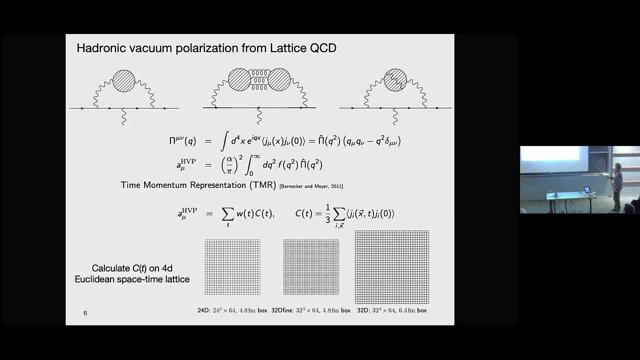 So on the lattice we're interested in, you know we're working with quarks and gluons, so you know there's actually two different types of diagrams that we need to calculate: so-called quark-connected diagram and the so-called quark-disconnected diagram, where the quark loops here are only connected by gluons. 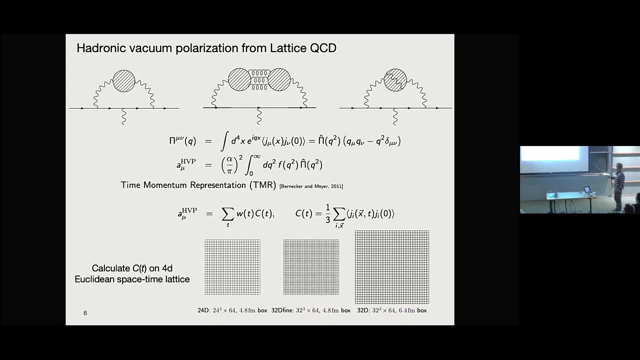 It turns out that this is by far the dominant contribution. This is mostly what I'll focus on today. We actually have to go one higher order in the fine structure Because if we want to compare to the data-driven result, we need these contributions, because they can't get rid of these in their analysis. 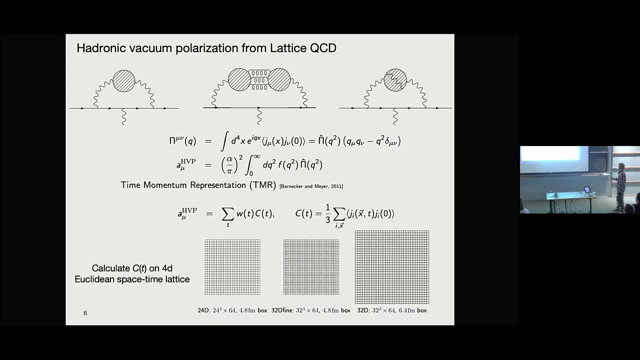 Okay, so for the lattice, we work in Euclidean time, Euclidean space, and it's much easier for us, instead of working in momentum space, to work in Euclidean space-time. Really, what we'll be interested in is the Euclidean time separation between two electromagnets. 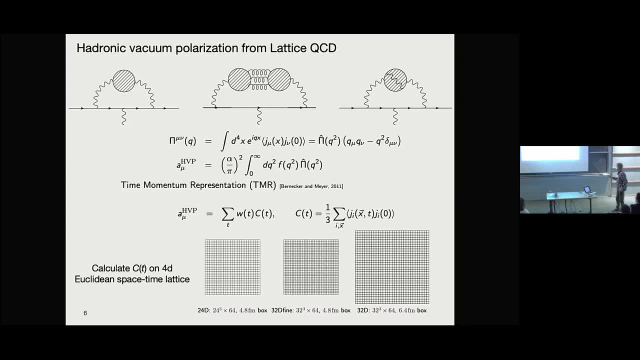 And you know just like you can get this contribution by doing this integral over momentum. well, in Euclidean time, we just have to integrate over the Euclidean time, Where, again, what we're going to measure on the lattice is this correlation function for the electromagnetic currents, but in Euclidean time, and then multiply it by some known function that comes from the QED part of the diagram. 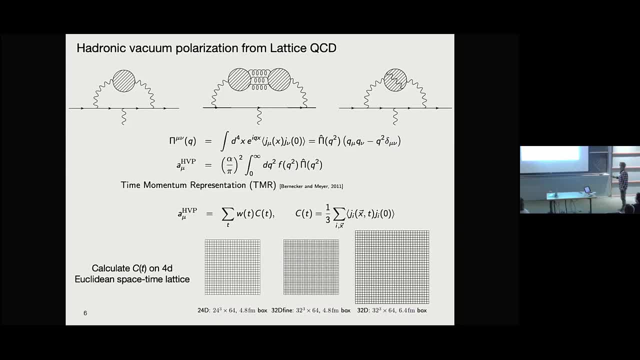 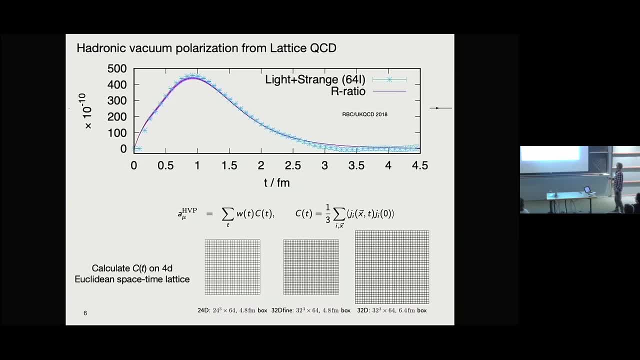 And this is just a typical example of what that looks like in a lattice calculation. So the blue points here are the lattice values, The magenta band here comes from somebody's calculation of the R ratio And the points to keep in mind are: you know, in a large range of Euclidean times the lattice does quite well. but as we get to large times, fluctuations from the dominant two-pion state mean that the lattice does quite well. 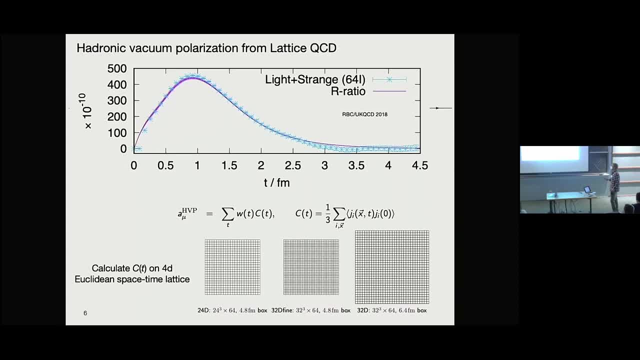 And so, you know, the correlation function becomes noisy, and so that's hard to deal with, And also at very short times. of course, you know, the vacuum polarization realizes: hey, I'm on a lattice, I'm not in the continuum, and there are big discretization effects. 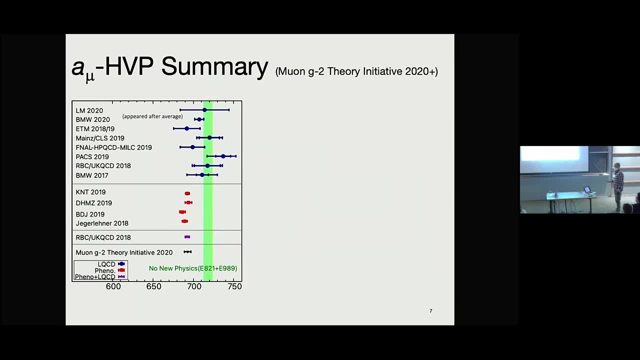 So here's the lightning summary of where the hedronic vacuum polarization contribution stands, And you know this basically comes from, again, the muon g minus 2.. So this is the theory initiative circa summer of 2020.. 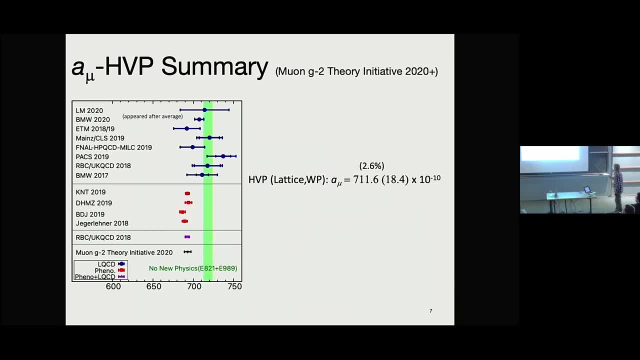 At that time this was the lattice value, which has a fairly respectable error, but you know it's still relatively large. And this should be compared to the data-driven approach, which comes in at a central value that's somewhat smaller than the lattice average and a much smaller error. so about a factor of four here? 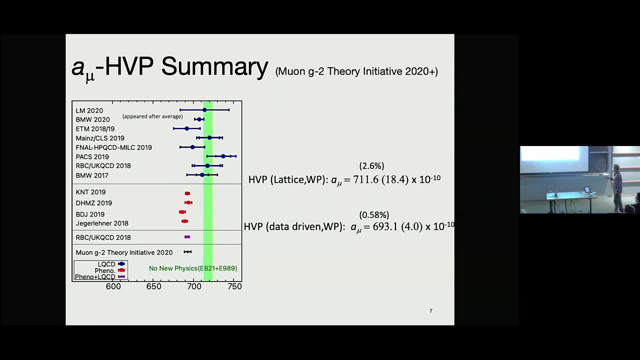 And so the lattice average comes from these blue points here, And the data-driven ones basically come from these two red points here at the top, with a little extra from some other areas. And then, after the white paper was published, one lattice collaboration- the BMW collaboration- came along with a lattice calculation with a quoted error that's on the same order as the data-driven approach, but still with a somewhat higher value. 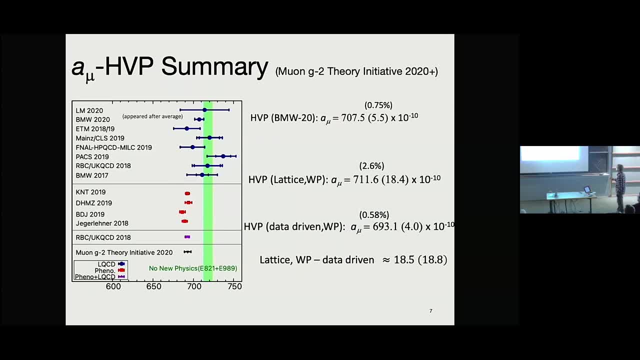 And so if you take the data-driven approach, you'll see that the lattice average is a little bit higher. And if you take the difference between the lattice value and the data-driven value, everything is completely consistent. And if you take the difference between BMW and the data-driven value, then things are off a little bit. 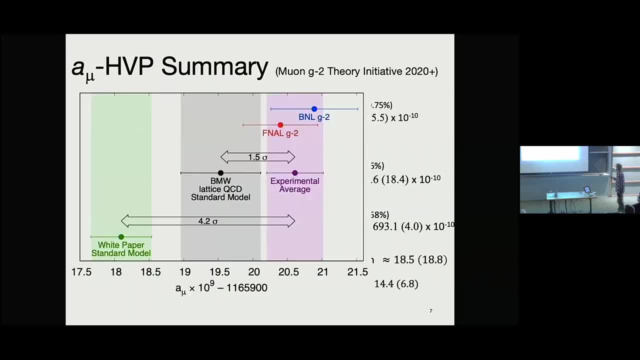 There's some tension here. But then if you compare those to the experiments, of course, what you all know is, if you take the white paper value and the data-driven HVP, you get a 4.2 standard deviation difference with experiment. 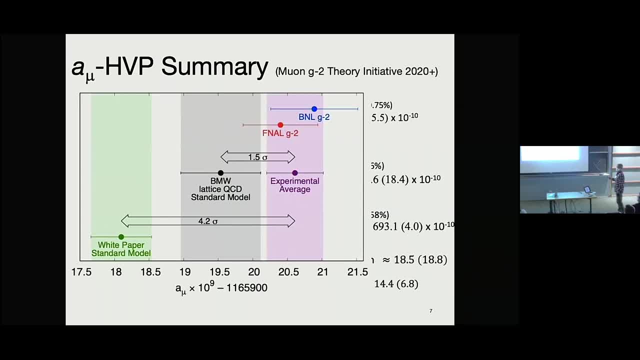 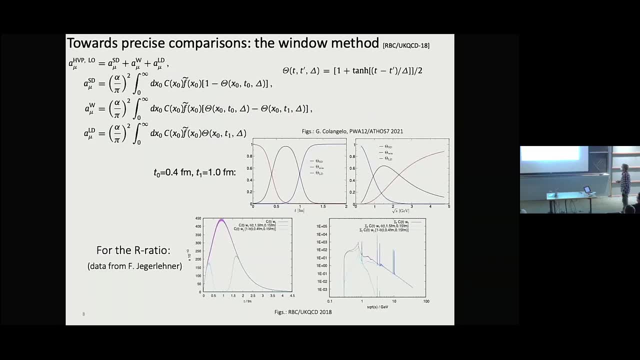 Whereas if you take BMW, it's only 1%. And so that's where we are now and that's what we're trying to understand. So to do that on the lattice side, what we're going to do is we're going to break up the problem into smaller chunks and attack the easy ones first and leave the harder ones for later. 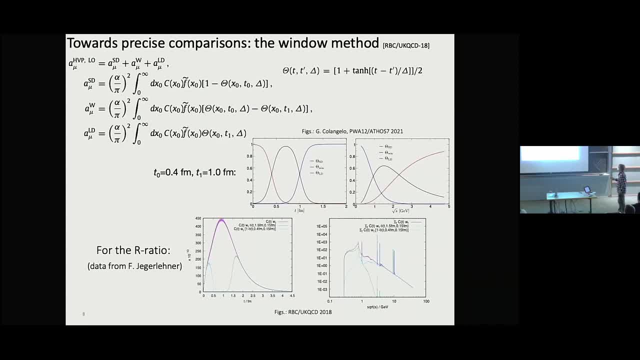 And so what we're going to do is we're going to break up that sum over Euclidean times into three chunks: A short distance piece, an intermediate piece, An intermediate distance piece and a long distance piece. And we do that just by inserting a smooth step function or filter into the integral which cuts off the regions we don't want and leaves the regions we want. 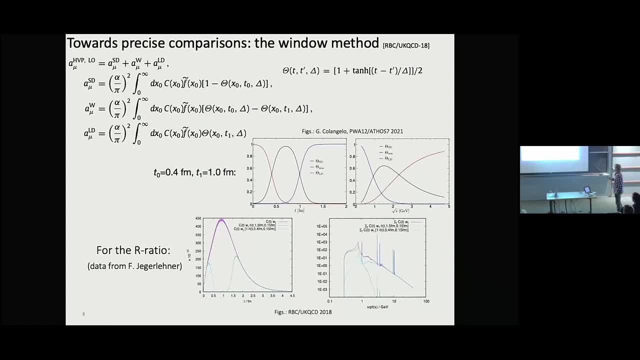 And that's what these windows look like. So there's the short distance window, There's the long distance window, And this is an intermediate distance window And this is what they look like in momentum space or energy space. And so, if you did that for the R-ratio data, 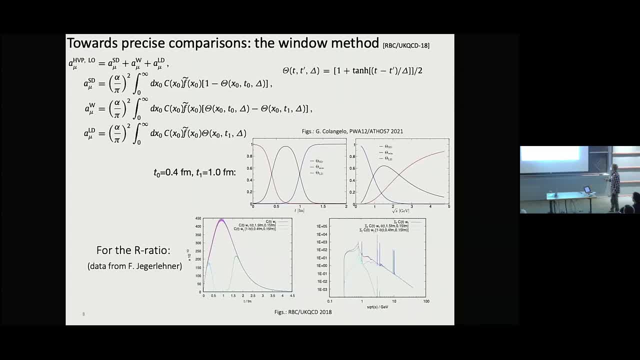 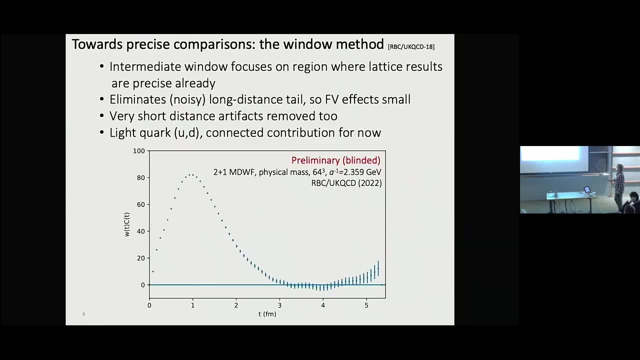 Again you have the total and you have the short distance contribution and then you have a long distance contribution And again it looks like this in energy space. So again, the reason we're doing that in the lattice is because we can do this intermediate range much easier right now than we can this long distance part where the fluctuations are quite large. 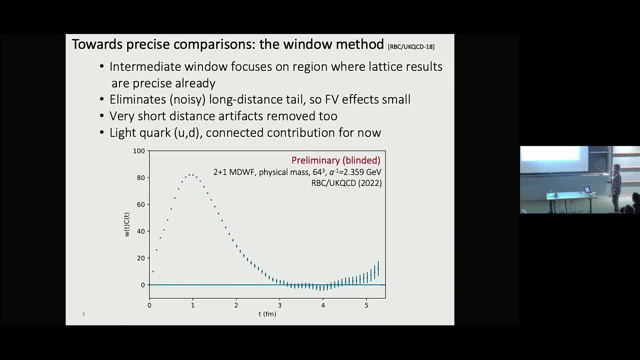 And again the short distance part where taking the continuum limit, Where the lattice discretization errors are quite large. And this is again the same sort of figure I showed, but it's new, updated data from the RBC collaboration. So let me start with so-called staggered fermions. 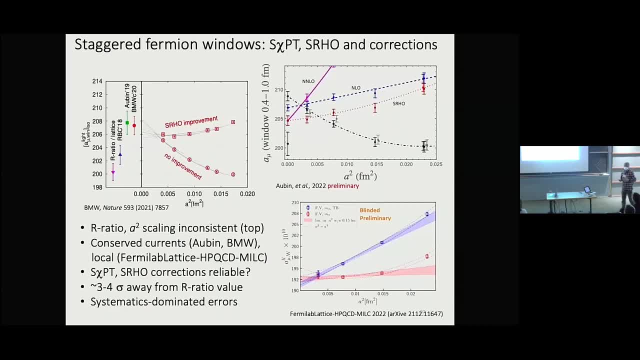 For those of you who aren't familiar with lattice fermions, they come in different shapes and sizes, And staggered fermions have the benefit that they're Expensive relatively to use, but they have a drawback: that they have extra degrees of freedom than you have in the continuum called tastes. 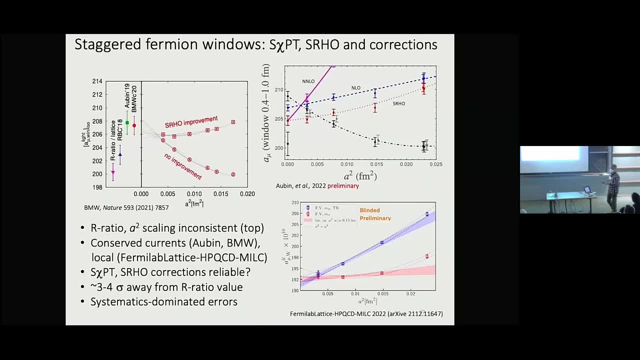 Because they actually come from the doubling problem. They're like extra flavors, but they're called tastes. And these tastes, their contribution, vanishes in the continuum limit, But at finite lattice spacing they can have quite large contributions that we have to account for. 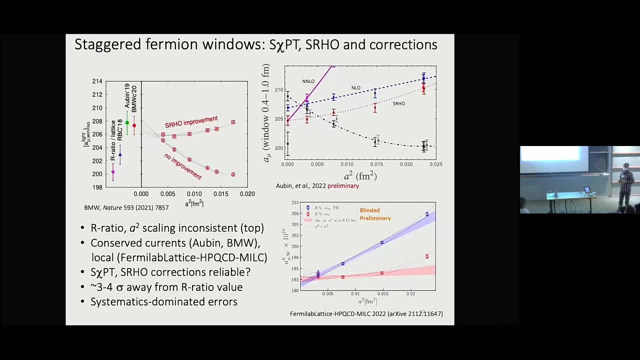 And so it's typical in lattice calculations. So we use these calculations with staggered fermions to actually calculate the taste-breaking effects in effective field theory, And even effective field theory plus models that include a vector meson, And subtract them before you take the continuum limit. 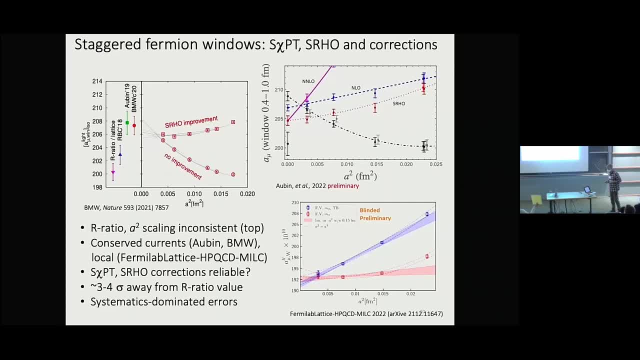 And then the idea is that taking the continuum limit will be easier. So this is the BMW collaboration's calculation of this short distance window: The contribution to a mu from the range, say, 0.4 Fermi to 1 Fermi. 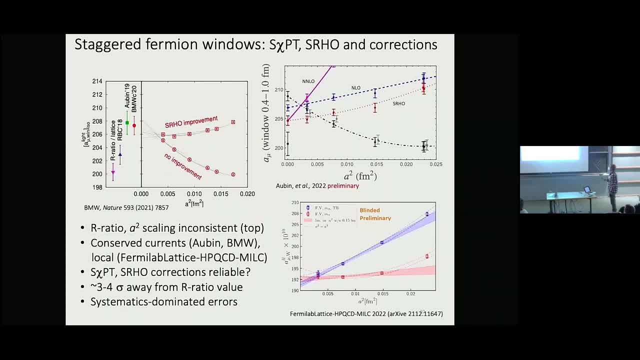 And this was the situation around the time of the white paper. So here's the R-ratio value for the window And here's BMW, without doing these taste corrections, And they extrapolate to some, you know would extrapolate to some rather high value. 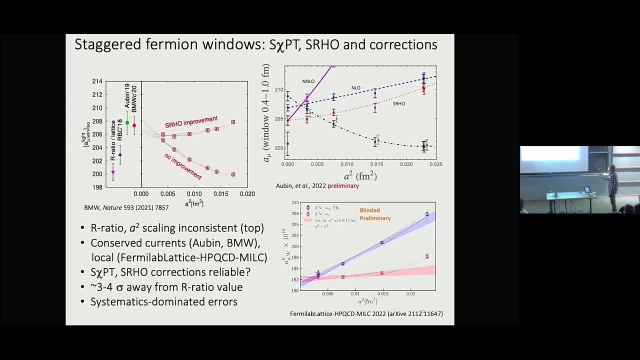 And then, with the taste-breaking, you see the lattice discretization effects appear to be smaller, but they're still not zero, And so when you extrapolate, you get some number up here, And this number is about four standard deviations different from the R-ratio value. 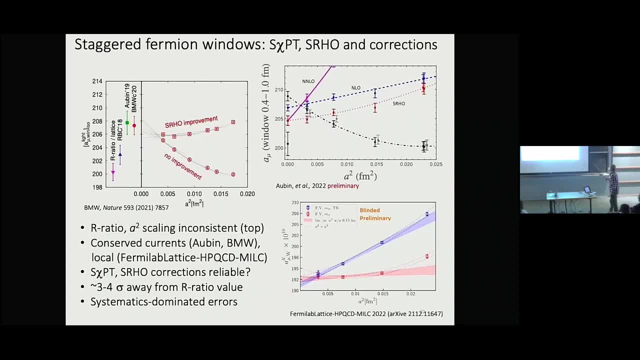 This is another collaboration using staggered fermions. And again, here are the uncorrected data in black, And then various corrections, the so-called SRO model, And then, next to leading auric hydroperitoneum, next to leading auric hydroperitoneum perturbation theory. 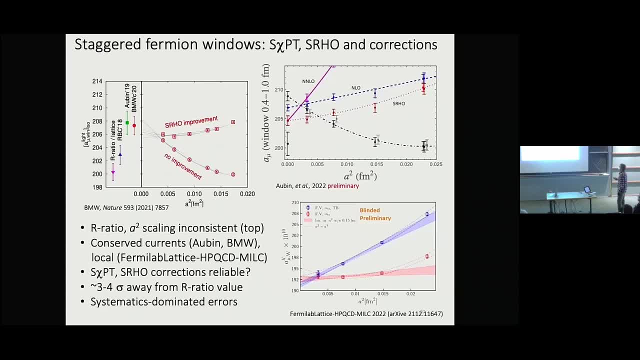 and next to next to leading auric hydroperitoneum perturbation theory, And again they give somewhat different answers, but they don't seem to agree with the R-ratio value. And then, finally, there's an update from the Fermilab lattice: HPQCD and MILK collaborations. 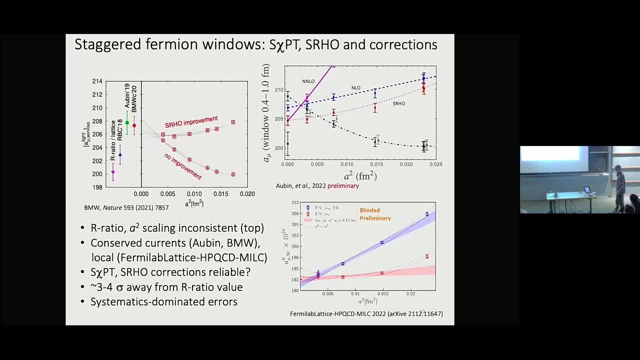 By the way, these two collaborations are using the same lattices and almost the same Dirac operator on the lattice. And they're using the same lattice and almost the same Dirac operator on the lattice, But they're slightly different. And here they're using conserved currents for the vector for the electromagnetic currents. 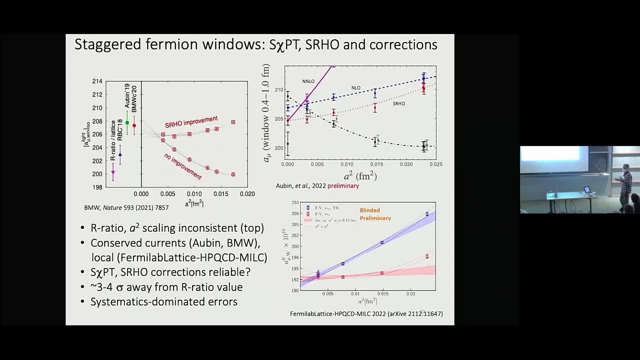 And here they're using so-called local currents that aren't exactly conserved on the lattice. But those are details, So it means that they can have different order A-squared effects, but they have to agree in the continuum limit if everyone's doing it right. 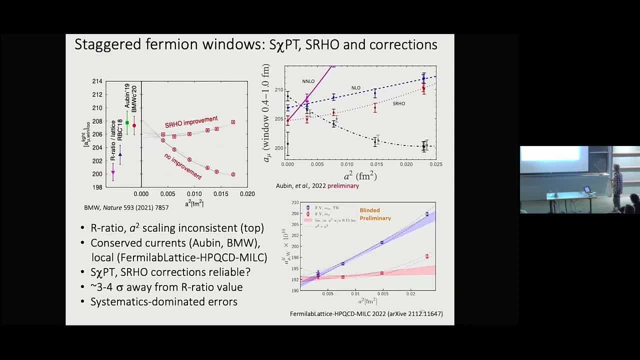 Okay, so this is the new updated value from FHM And they have quite small errors, but at the moment they haven't unblinded, So we don't know if this really is going to be consistent with these staggered calculations or consistent with the R-ratio. 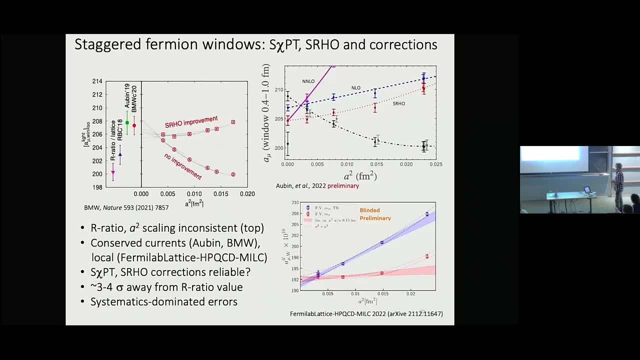 And one of the important things to notice here is that we're systematics dominated at this point through the window, not statistics dominated. And the question is: are these corrections really reliable At this level? Because you know, we need fantastic precision. 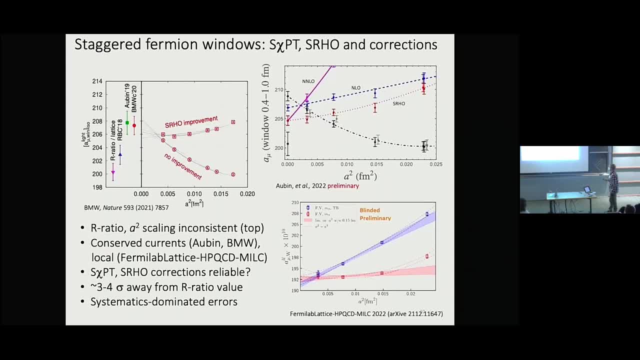 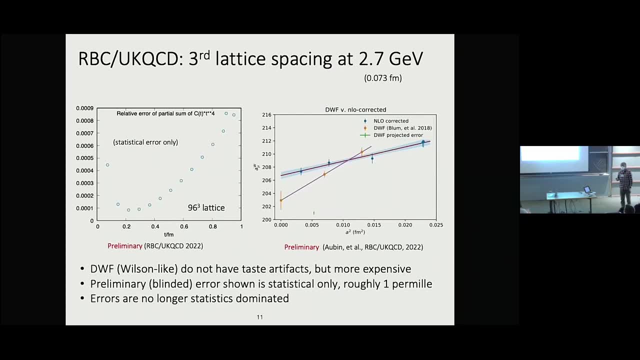 So those are the kinds of things that we're asking ourselves and looking into at the moment. Now there are some discretizations that don't have these tastes. They don't have tastes and so they don't have taste violations. Okay, good. One of them is the RBC collaboration. They use something called domain wall fermions which, if you know anything about lattice, are Wilson-like fermions. So there's no taste, but they're more expensive to compute with, So there's trade-offs. 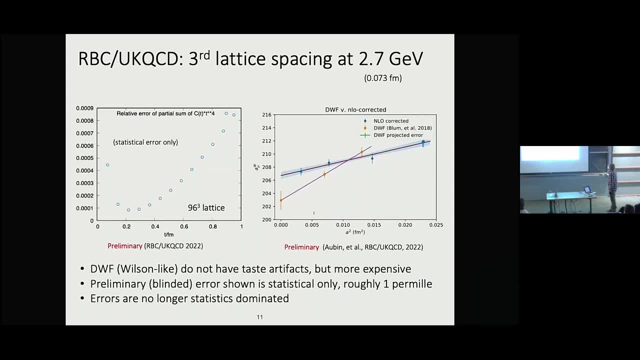 But you know it's again at the time of the white paper. the domain wall fermions, which were only done at two lattice basings so far, because, again because they're expensive, seem to be consistent with a lower value for this window quantity. 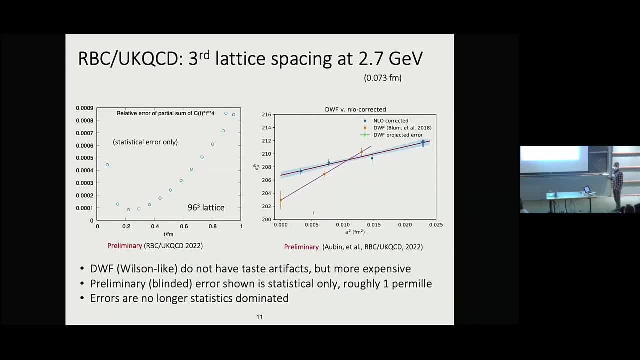 which in fact is consistent with the R-ratio value. So the question is: what happens when you add a third lattice? It's a smaller value. Is it still consistent? or, you know, does it become more consistent with the staggered fermion calculations? 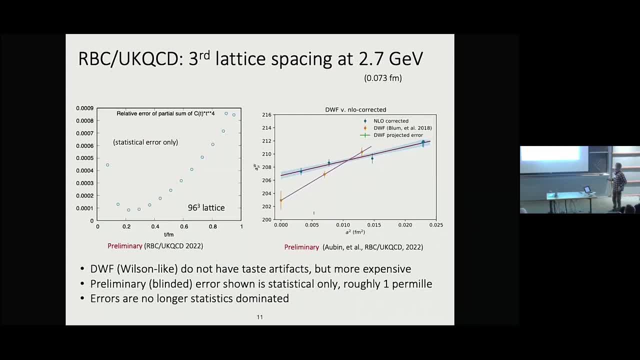 And we don't have the answer to that yet, but that's what we're really working on And in fact we do have an error bar for that calculation, and it's very, very tiny. It's on the order of a per mil. 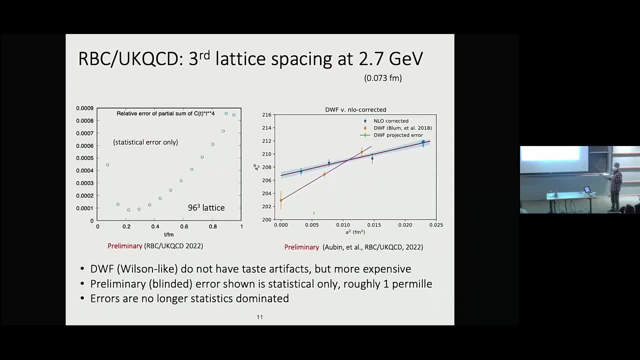 But again, this is an analysis that's ongoing and it's still blinded, so we don't know what the answer is yet. Hopefully very soon, And again, even for domain wall in this case. now you're no longer statistics-dominated. 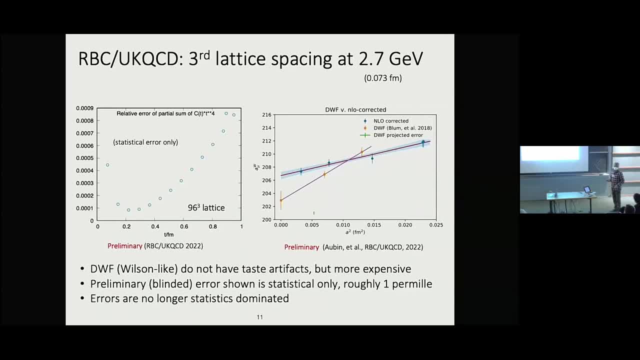 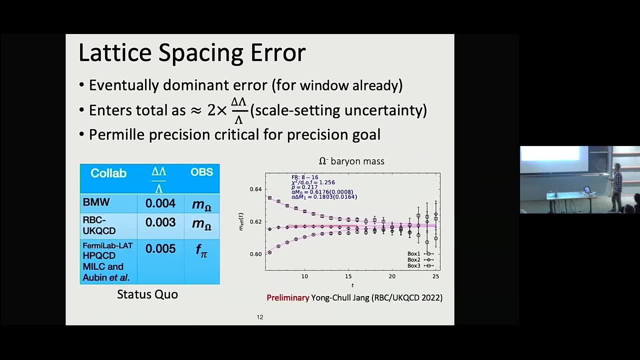 You're going to be dominated by systematics, Oops, Okay, No time left, So let me – this is my last slide, Because things are becoming statistics-dominated. it's also incredibly important now to be able to precisely determine things like the lattice spacing. 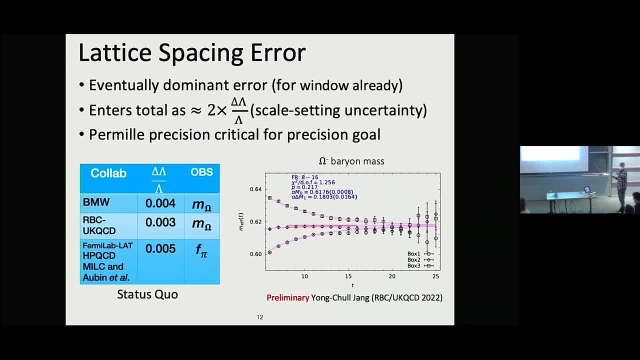 Not only to do the extrapolation, but the lattice spacing actually affects the value of a mu, because the muon mass, which is a physical scale, enters in this kernel function, And so the lattice spacing enters, and it enters about a factor of two times this scale-setting uncertainty. 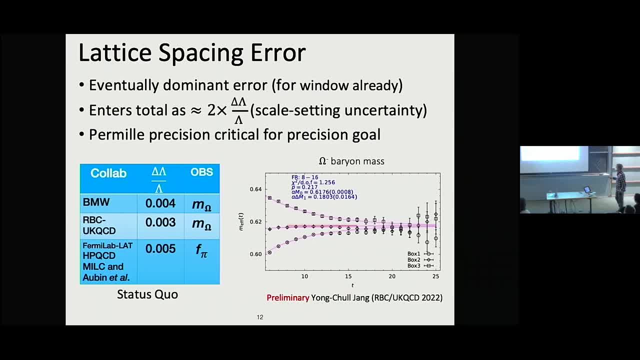 And these are sort of the state-of-the-art scale-setting uncertainties, and those have to come down as well To the per-mil level if we're going to reach our precision goals, And we're – you know, the RBC collaboration, for example, is on track. 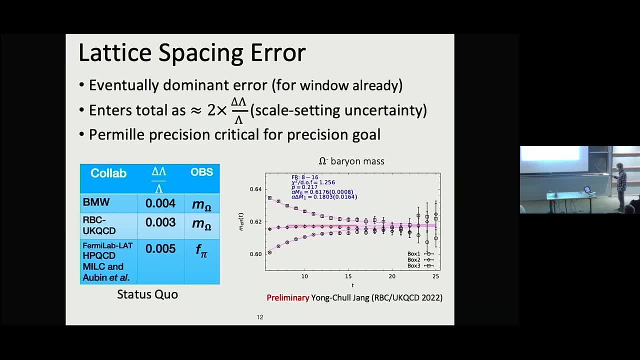 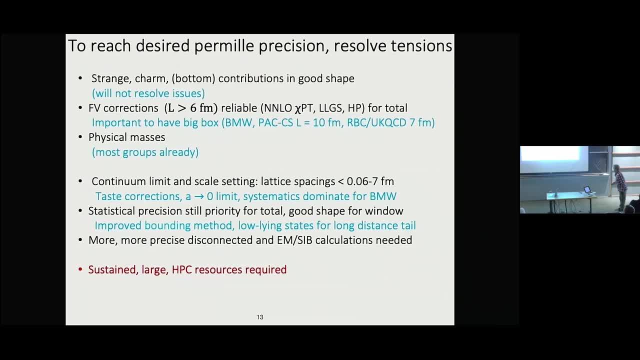 So this is – this will be a scale-setting determination on that fine lattice. that's about a per-mil. Okay, You know, this is just what I said. I didn't talk about this stuff, but since I'm out of time, 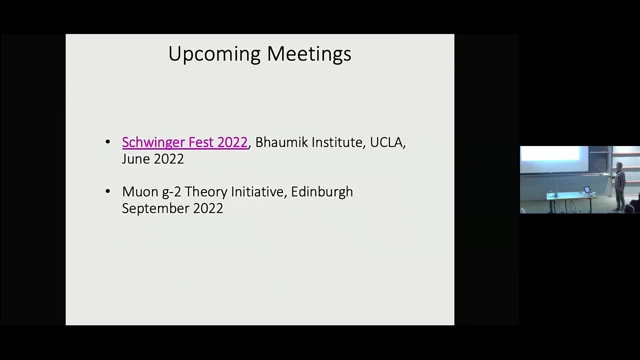 I'll just end with that, but also tell you that there are two meetings coming up this year where, hopefully, new results will be announced. So you know, keep your ears open, you know, around June and maybe in September. So thank you very much. 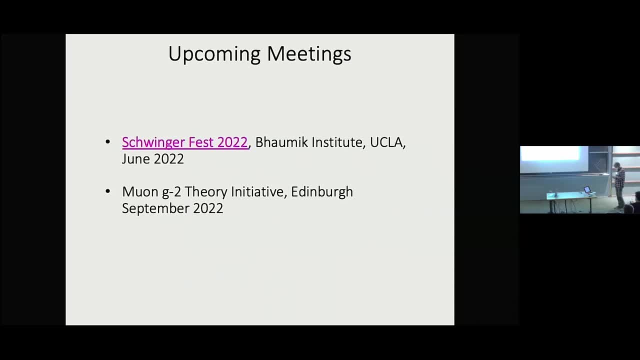 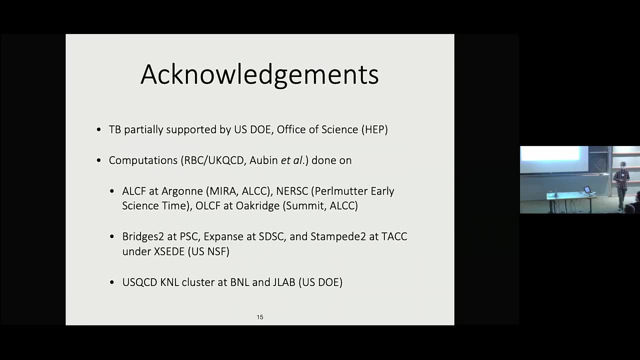 Thank you, Tom, for this very clear talk. Are there questions from the room? I can't resist making a stupid comment. The one time I encountered Schwinger, he railed against the stupidity of QCD with quarks and gluons. 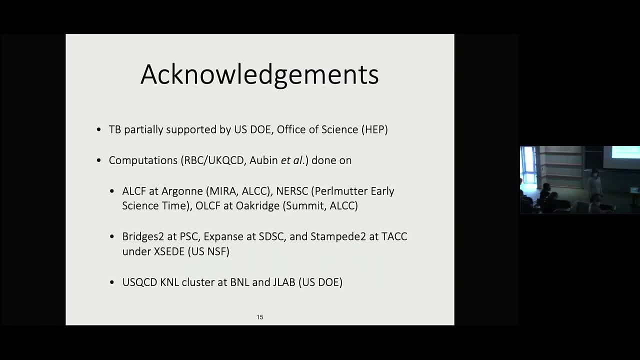 How could anybody believe that? So, when you talk about this, at his celebration of the anniversary of his birth, is he going to roll in his grave? He's not going to roll, He's going to precess. Can I ask a question too? 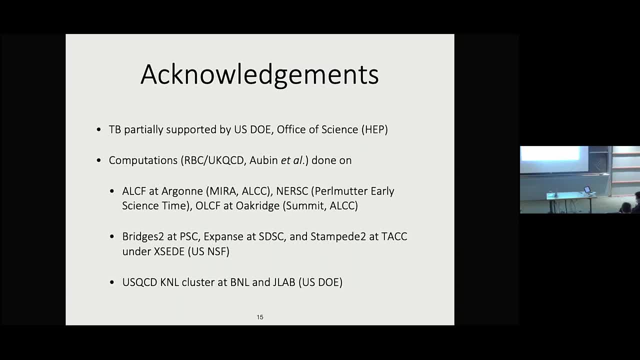 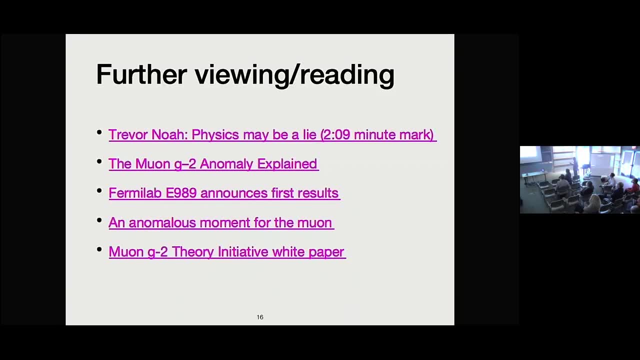 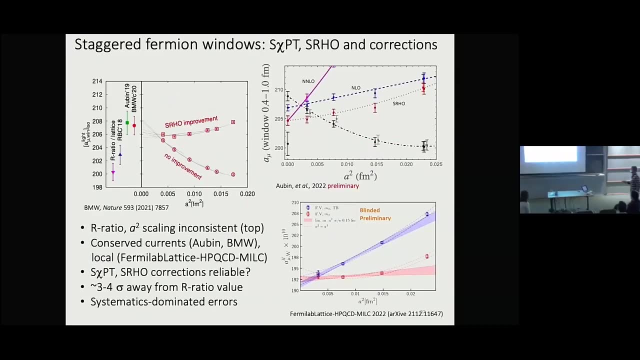 Sure, Sorry. this is Lance Dixon. You showed a plot there that showed extrapolations for NLO and NNLO, Right Chiral perturbation theory, and NNLO is steeper than NLO. Should we be worried about this? Yeah, I mean that goes to this question about you know, are they reliable? 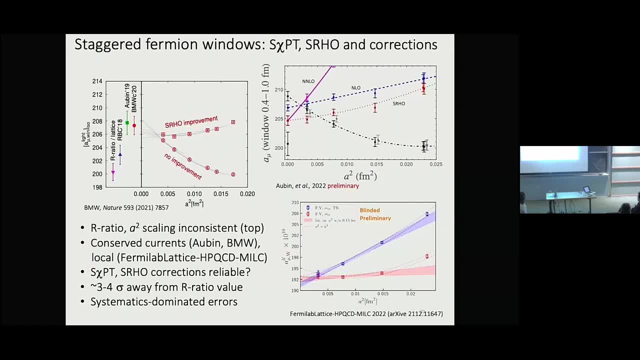 So here there's a good reason for this big jump from NLO to NNLO, because at that point the Rho meson comes in from a counterterm in NNLO which is not there in NNLO. So that's why the big jump is there. 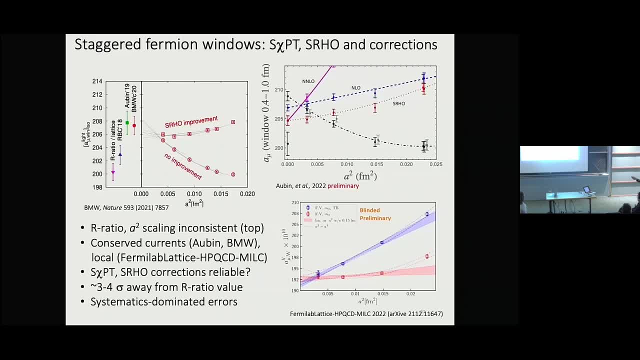 But you know, for this window, from the point of view of chiral perturbation theory you could say it's kind of a short distance quantity, Because you know you go down to fairly short distances And so chiral perturbation theory may not be reliable. 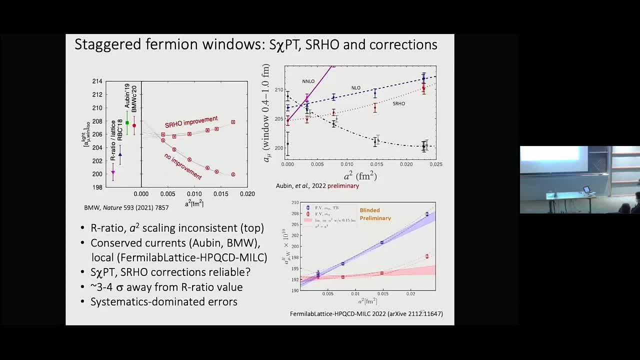 Thanks. There's good reason to believe it's reliable for the entire contribution. Hi Tom, This is Aida Al-Khadra And I just wanted to follow up on this discussion, As I know you agree as well. What is important about chiral perturbation theory? 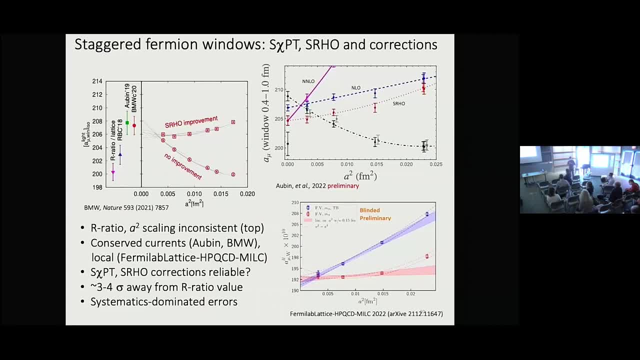 And also making sure that those corrections are well understood, is to see that, whether or not you add these corrections, if you are in the range where these are small enough that you see that there's consistency between the continuum limits And you know if there's not consistency, then that has to inform the error, the systematic error, which is the point that you were making. 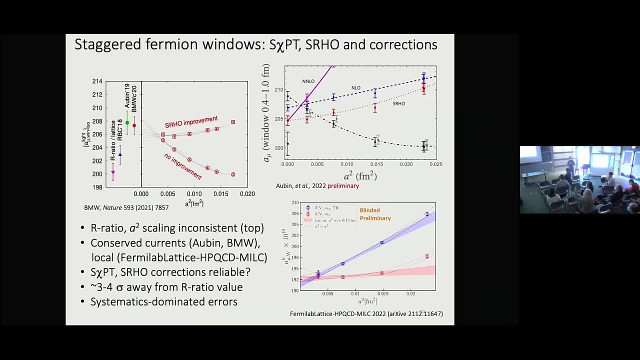 Yeah, I mean that's. the claim for BMW is that they can actually, for the intermediate window, they can extrapolate their data without including the corrections, And the concern is that for the total AMU they cannot do that because their taste breaking corrections are so large that they're not describable as just AMU. 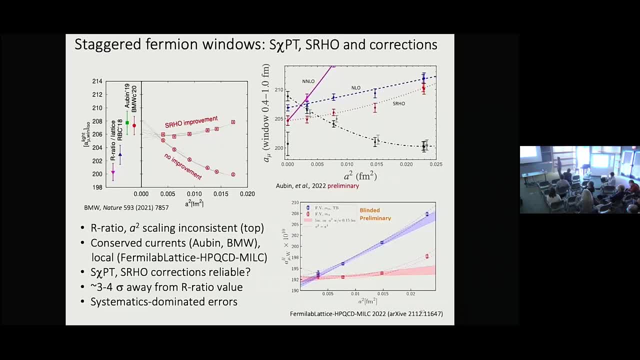 Yeah, I mean you can see that in their flavor of pardon the pun of staggered fermion, you know it's just larger. So I think there's a lot to be learned just from having different flavors of staggered fermions as well to really understand that. 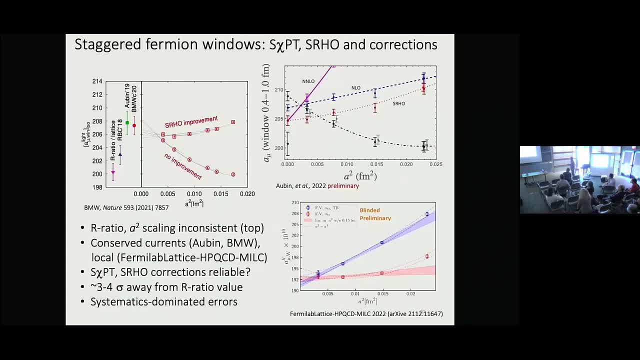 It's hard to tell from this plot, but it looks like, if you extrapolate the uncorrected data, right, Yeah, It's even quite a bit higher than the. I don't know if these are consistent or not, but you say in their paper: they say they are. 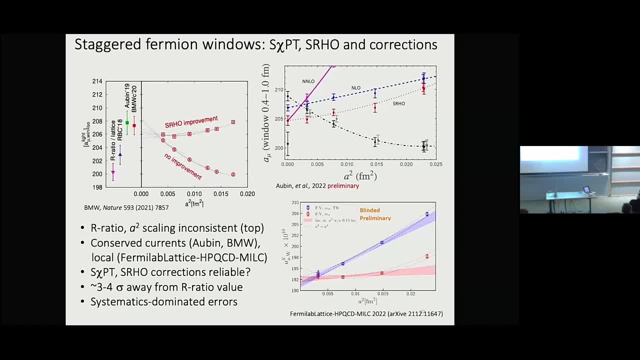 To me it looks a little problematic, But I you know. I would just add to what you just said that for BMW, their largest error, part of their error, comes just from this. you know the difference they get depending on how they do the corrections. 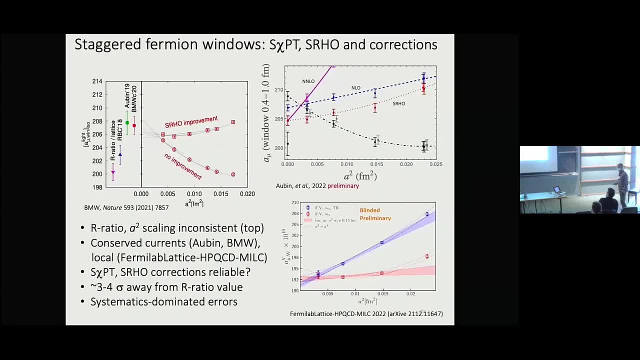 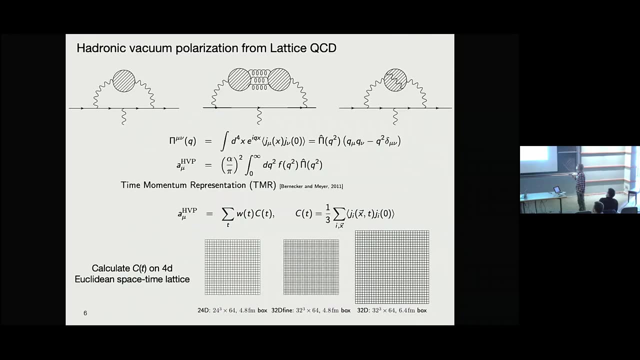 Hi Patrick Mead. If you go back to the diagrams that you are computing for the lattice, you mentioned that you have to go for HVP one order higher to kind of match the data driven in the weak coupling. But can you say a little bit more about this? 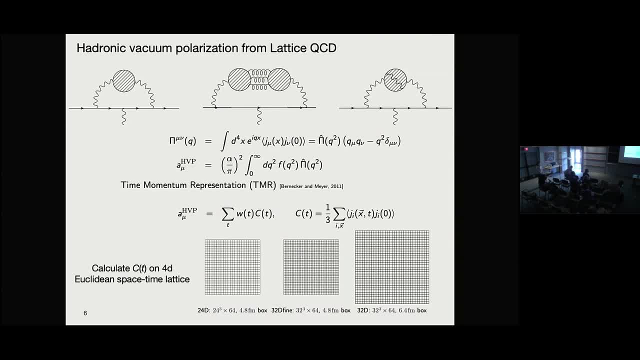 Is it just the standard model measurement? Is it trying to move as much of the ISR as possible? And I mean, there's still this ambiguity, but This isn't that ambiguity. Okay, so that's not that ambiguity. This is just a real contribution that they can't get rid of. 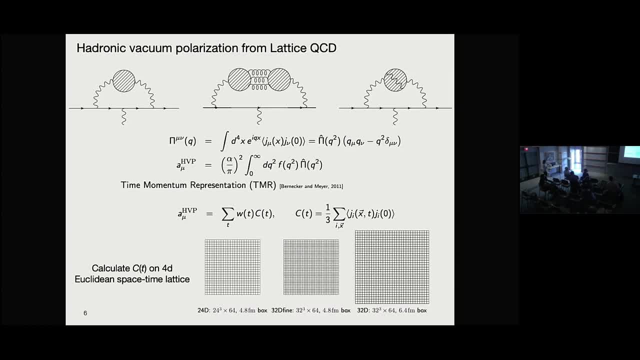 Okay, Yeah, Okay, Thank you. Just very quick question. I was actually wondering if you could hear your thoughts about the how do you get back in polarization contribution and the recent discussion of the fact that the tension between standard model measurements might be reduced. 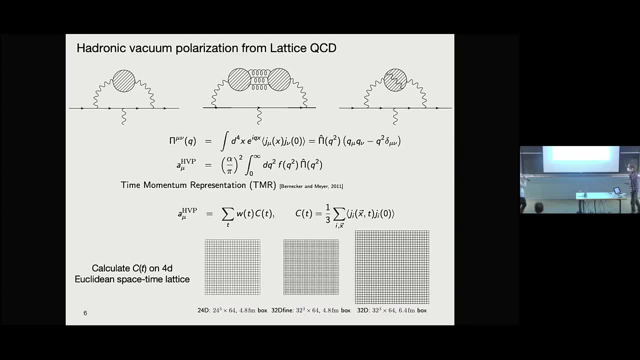 I was thinking maybe you can share your thoughts. Sorry, reduce because why The hydronic vacuum polarization contribution to NEON G-2 and the fact that the tension between standard model and data is potentially reduced? There was this paper from 2020 on the topic.